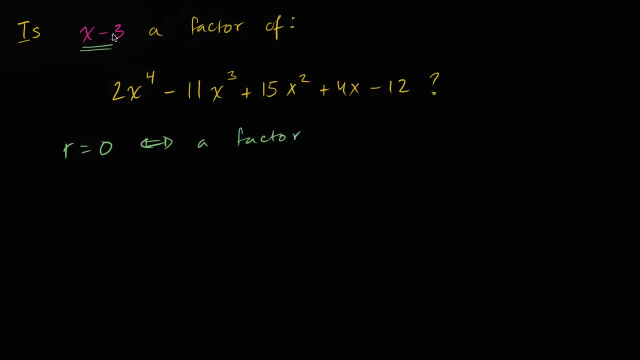 by a first degree polynomial like this, The polynomial remainder theorem. the polynomial remainder theorem tells us that if we take some- let me do this- some polynomial p of x and we were to divide it by some x minus a, then the remainder is just going to be equal to. 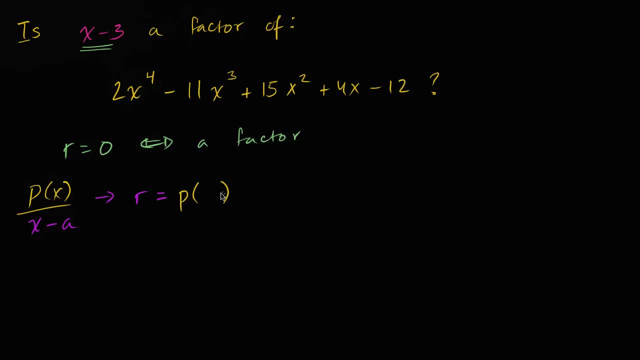 our polynomial evaluated at our polynomial evaluated at a. So let's just see what's a in this case. Well, in this case, our a is positive three. So let's just evaluate our polynomial at x. equals three If what we get is equal to zero. 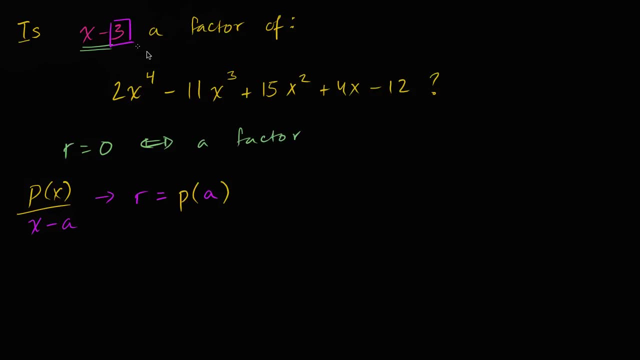 that means our remainder is zero and that means that x minus three is a factor. If we get some other remainder, that means well, we have a factor. that means well, we have a non-zero remainder and this isn't a factor. 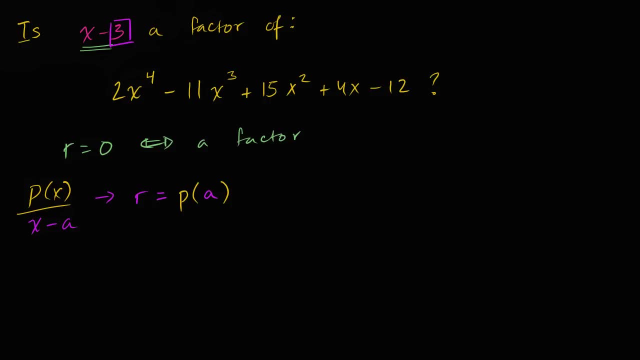 So let's try it out. So we're going to have, so I'm just going to do it. I'll do it all in magenta. It might be a little computationally intensive. So it's going to be two times three to the fourth power. 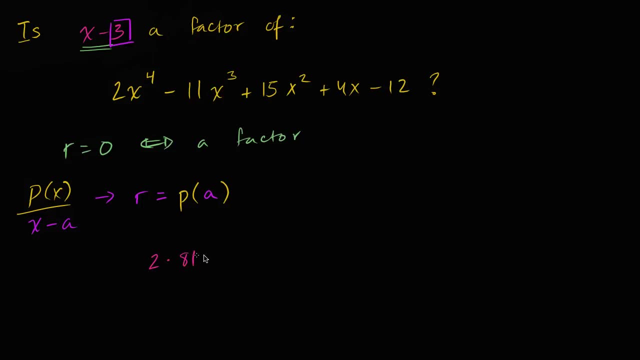 Three to the fourth, three to the third is 81.. 81 minus 11.. Yeah, this is going to get a little computationally intensive, but let's see if we can power through it. 11 times 27.. I probably should have picked. 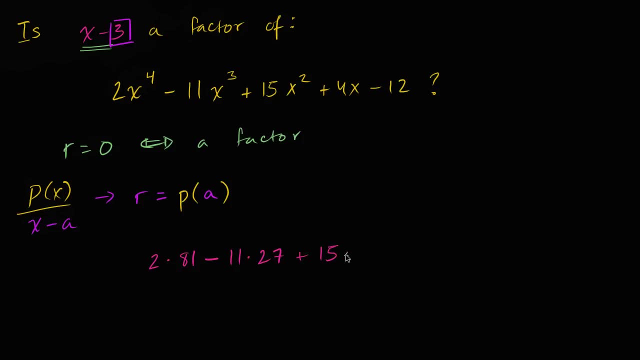 a simpler example. but let's just keep going. Plus 15 times nine, plus four times three is 12, minus 12, so, lucky for us, at least those last two terms cancel out, And so this is going to be. 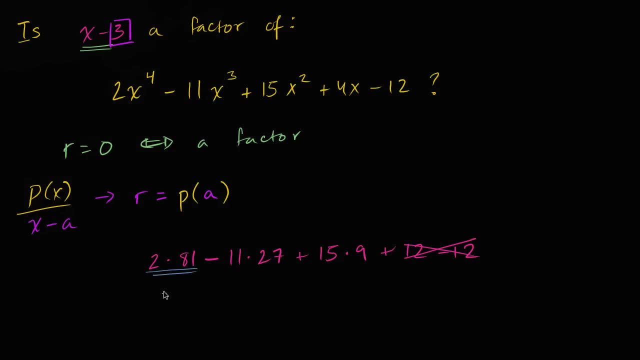 the rest from here is arithmetic. Two times 81 is 162.. Now let's think about what 27 times 11 is. So let's see, 27 times 10 is going to be 270.. 270.. Plus another 27 is minus 297.. 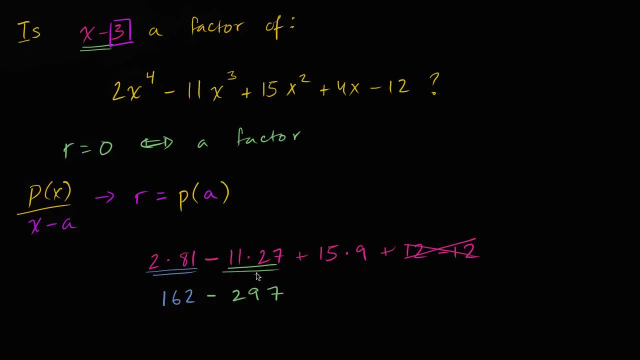 297.. Did I do that? Yeah, 270.. So 27 times 10 is 270, plus 27, 297,. yep, that's right. And then we have- I'm prone to make Carol Sowers here.